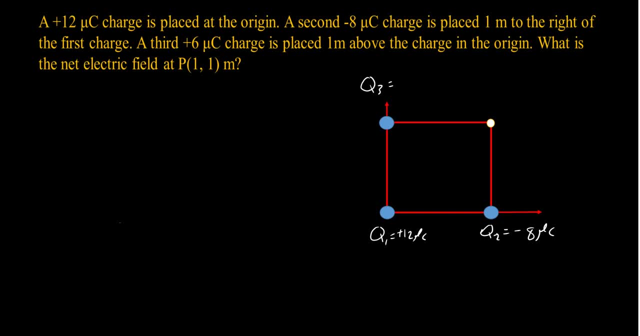 have Q 3, which is the positive 6 micro column above the origin, one by 1 meter. now this is the point B- will be here the coordinate 1, 1 meter. so I know the distance between the two charges and I know the distance between the two charges. 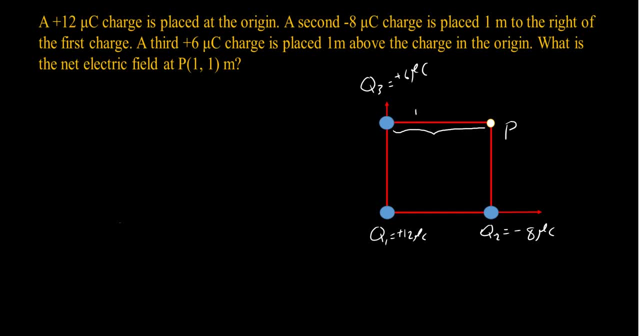 between Q 3 and point B will be one meter and the distance between point B and Q 2 will be also a meter, and by calculating the distance between Q 1 and point B, it will be square root of 2. let's start calculating the electric. 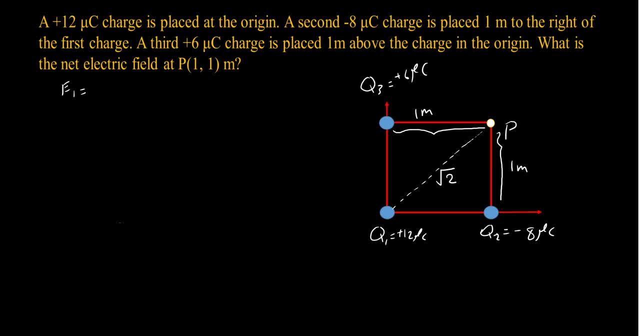 field 1, and it is K Q 1 over R 1 square, that will be 8.9, 10 to the power, 9 multiplied by 12, 10 to the power minus 6. all divided on the distance square, that should give me 53.6. 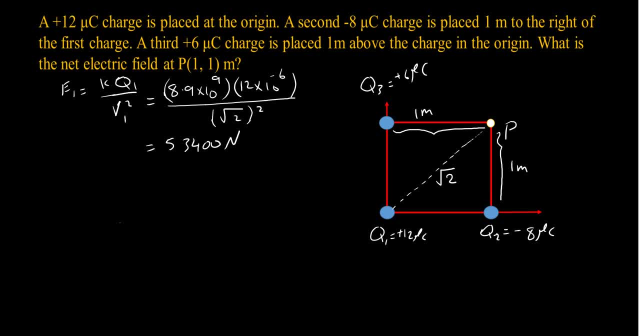 thousand four hundred Newton per column. now to decide the direction or identify the direction of the electric field 1, it will be. we have a positive charge, Q 1, and the electric field at point P will be away from it. so this is the direction of E 1. let's calculate E, the electric field generated by the second charge. we. 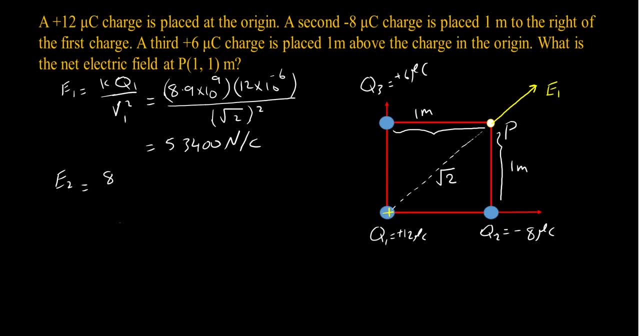 fill the charge and some other reaction. nu, if we enable and we have the flux constant, J just generated from the surge point, we have due charge, Cu transmitted. we will go to the average voltage from E and we will follow the same formula above and it will be 8.9. 10 to the power 9 multiplied by 8. 10 to the power minus G not faded to the power 9 multiplied by 8, 10 to the power minus. 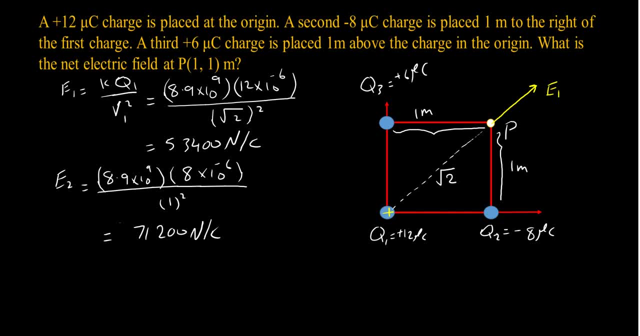 identify the direction of the electric field. well, q2. as we can see, it's a negative. so the electric field at point B will be going in or toward the direction of q2. so that will be our electric field, which means I can place a negative value here to represent the direction. and to the negative. 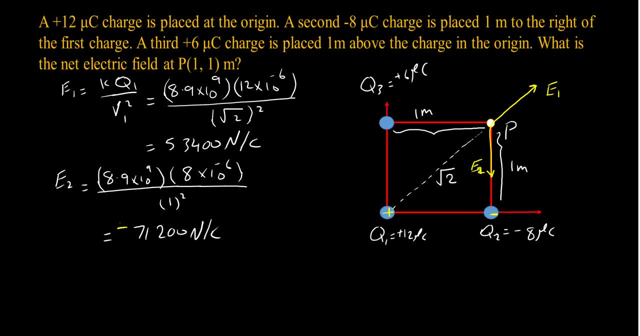 y-axis. okay, now let's calculate. and the electric field generated by the third charge. it will be eight point nine, ten to the power nine multiplied by six, ten to the power minus six, and all over the distance squared, and that should give me fifty three thousand and four hundred Newton per column. and to identify the direction of, 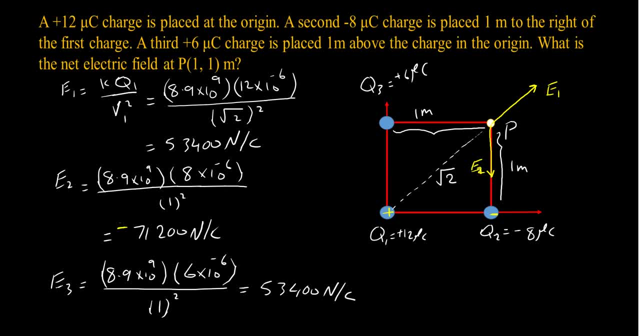 the electric field generated by q3. it's a positive charge, which means it's going to be going away from it at point P. that will be our electric field. it's right? okay, so now we we managed to calculate the magnitude for every single electric field generated by. 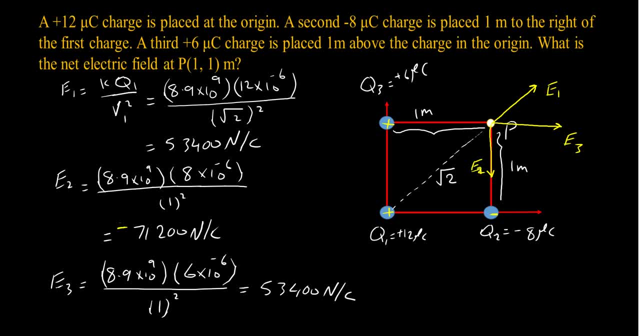 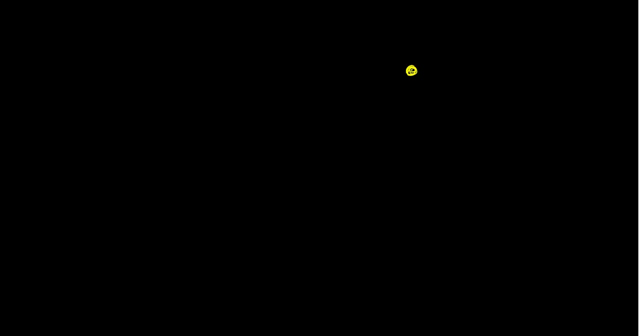 every single charge at point P. now to calculate the net electric field, we still need to do one more step, which is analyzing the electric field one into two components. and we have the angle here. it will be 45 degrees. okay, so what I can do, I can redraw the whole thing, and this is my point B, that's my 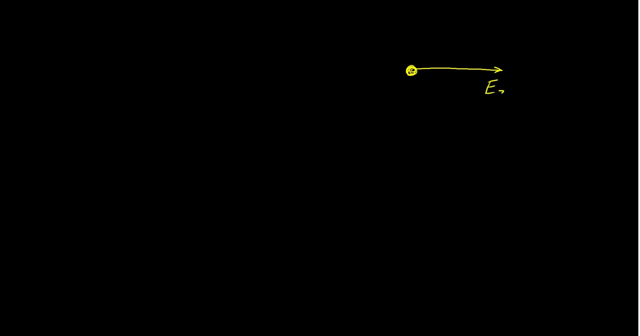 electric field three, that is my electric field one and this one will be my electric field. now I can. this is the angle we set, so 45 degrees, which means I can analyze the electric field one into two component. one will be electric field one, X- and also electric field one Y component, and I can do the math for each one of these. 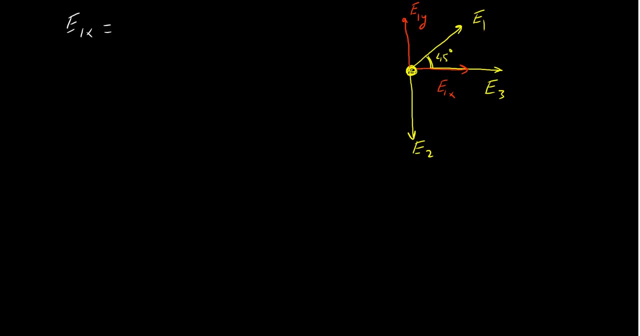 components. I say you 1, X. it will be the magnitude of e1, or the electric field, 1 cosine 45 degrees, and that should give me 37.75, 10 to the power, 3 Newton per column. for the Y component of the first electric field. I'll have e1 sine 45 degrees. it will be 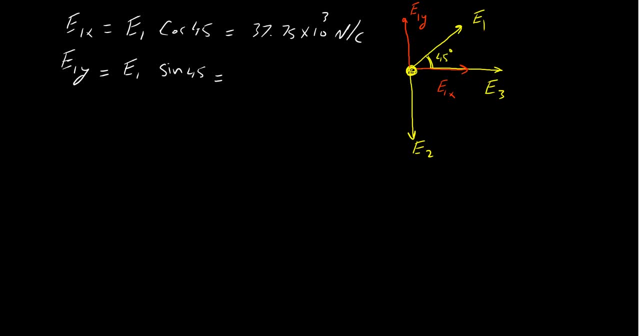 the same. all right, it will be the same value as a magnitude, 7, 5, 10 to the power, 3 Newton per column. so all right. now let's find out how much is the total electric field on the first electric field on the x-axis. so the total e X will be- I'm adding all the electric field. 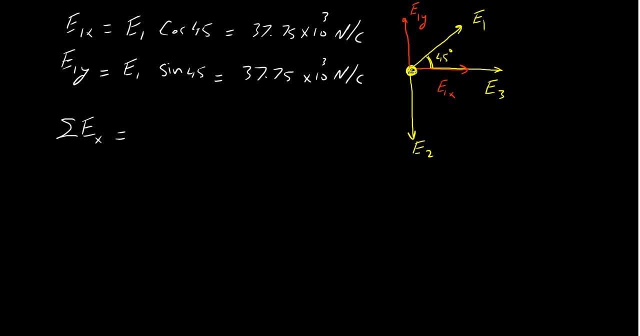 vectors on the x-axis. so I will have all these together, e1, X plus e3, and just doing the math for that it should give me 91.1, 5, 10 to the power, 3 Newton per column, and it's definitely going to the. 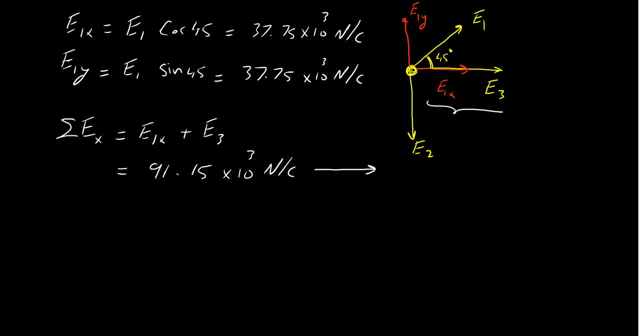 positive x-axis for the total electric field on the Y side or Y axis, I only have e1 Y component plus second electric field and if I do the math that will give me a negative 33 point or 5, 10 to the power, 3 Newton per column. and the negative helped me to say it is gonna be going to.